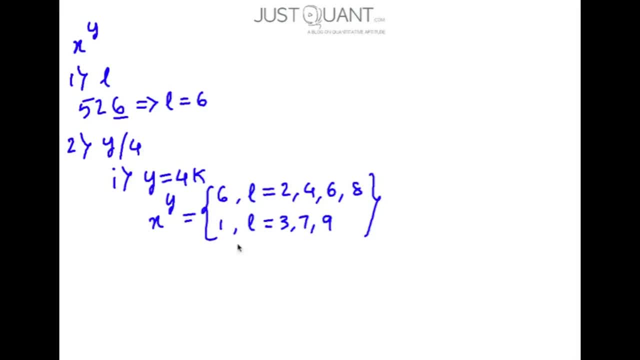 to the power of y will be equal to 1.. If l is equal to 5, then we will always see that the unit digit is 5.. So I will continue the case here In the next case where the value of y is. 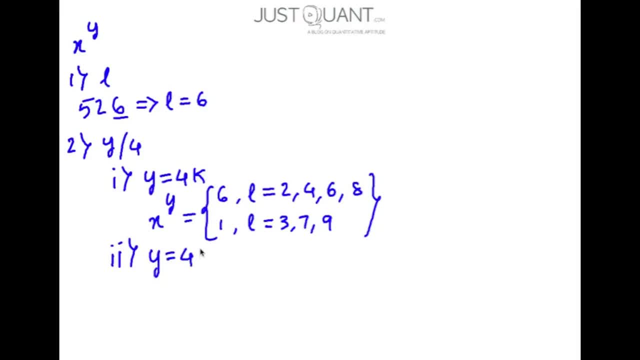 not exactly divisible by 4.. In that case we can write y as 4k plus r, where r is the remainder that we get upon dividing y by 4.. In such a case the value of x to the power of y will be equal to- I mean the value of the unit digit in x to the power of y will. 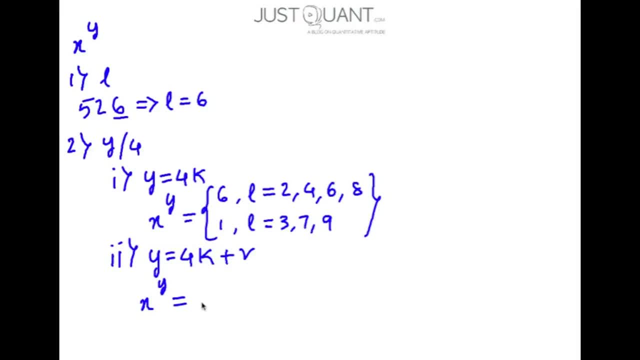 be equal to the value of unit digit in l to the power of r, where l is large digit obtained, or the l is the unit digit in x And r is the remainder that is obtained upon dividing y by 4.. Now, this will be clear if 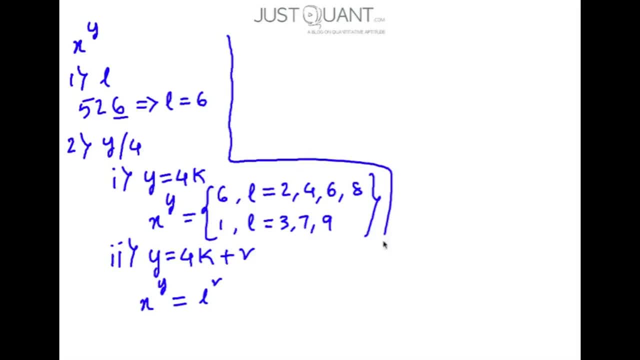 we saw some examples. based on these cases, I will consider taking the power of say I mean calculate- 74 to the power of 96. In this case we have the value of l, that is, 74, as 4.. And y, we see that is exactly divisible by 4.. 4 into 24 is 96. So we have to calculate. 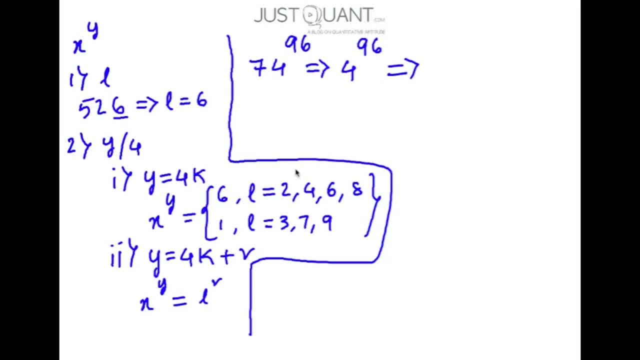 the unit digit of 4 to the power of 96.. So, as per our case here, since y is exactly divisible by 4 and the value of l is 4,, we will have the unit digit value as 6,, which is as per. 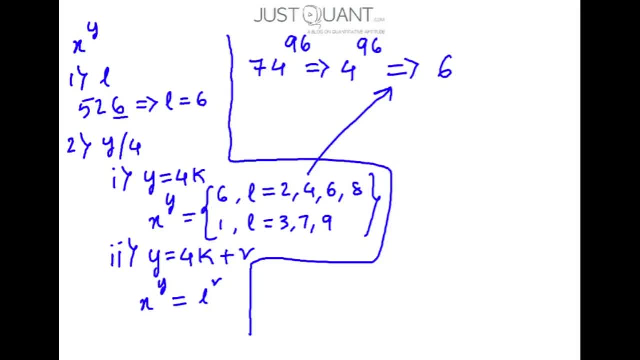 this case. In the next case, if I consider this as 73, we will have the unit digit of 4 to the power of 96. In this case, the unit digit in 73 is 3 and the power is 96. So this will be. 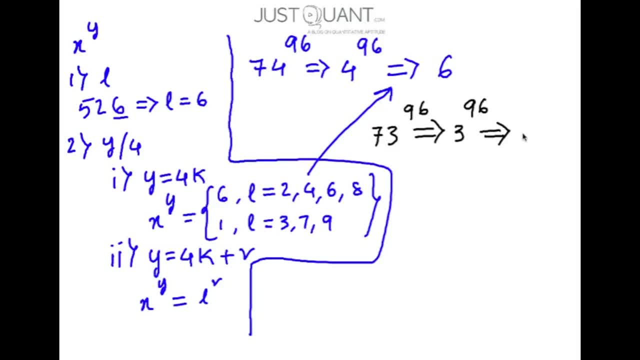 equal to this will give us 1 as the unit digit, which is as per this case. And then considering the case where you will try to calculate the unit digit of 97 to the power of 97. In this case we see that the value of y is not exactly divisible by 4. So y gives